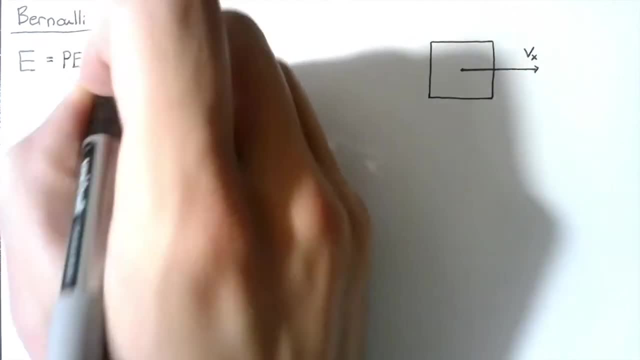 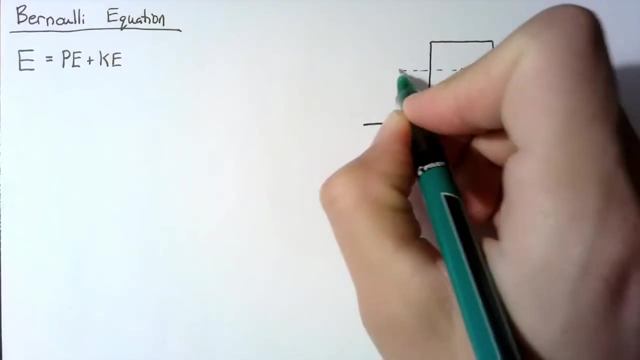 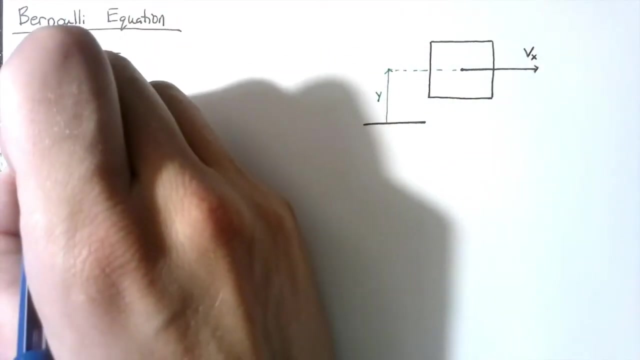 We're going to be focusing on the potential energy and the kinetic energy. The potential energy is based on gravity, so I'm going to say that this distance here is y, which means that the potential energy is going to be y. This is going to be the mass delta m of our differential element multiplied by gravity. 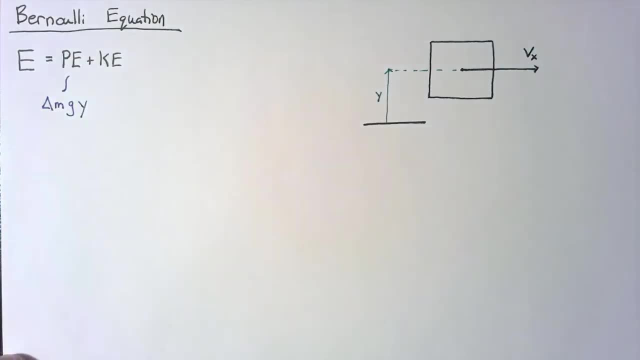 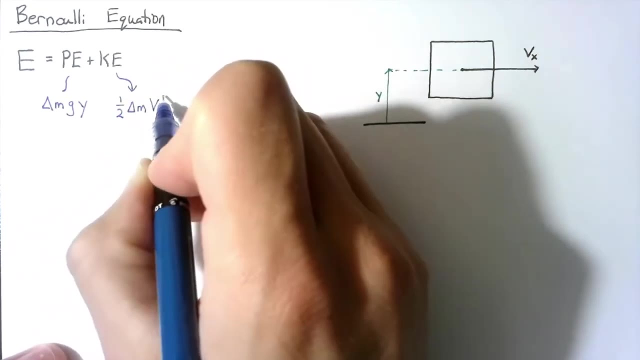 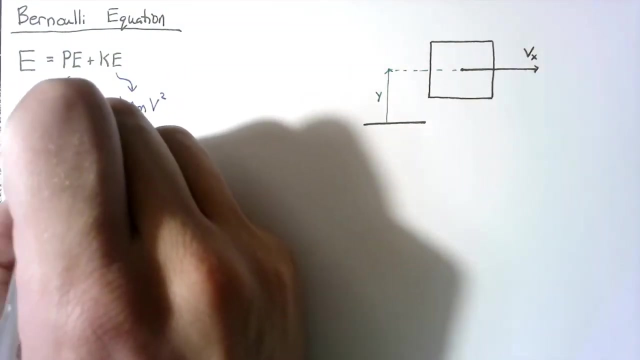 multiplied by the distance y from our reference point, The kinetic energy here is going to be the standard: one half times the mass times the velocity squared. This is how we're defining our energy for this fluid element. What we need to do next is look at the conservation of energy equation. 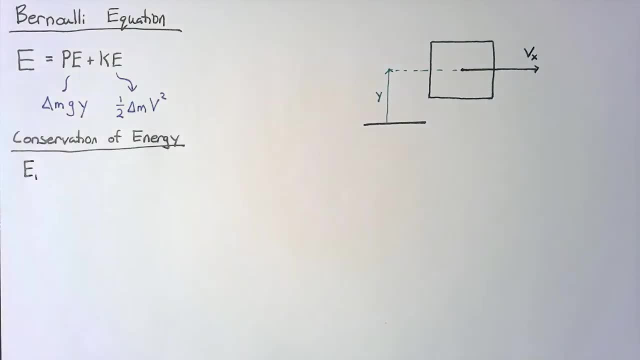 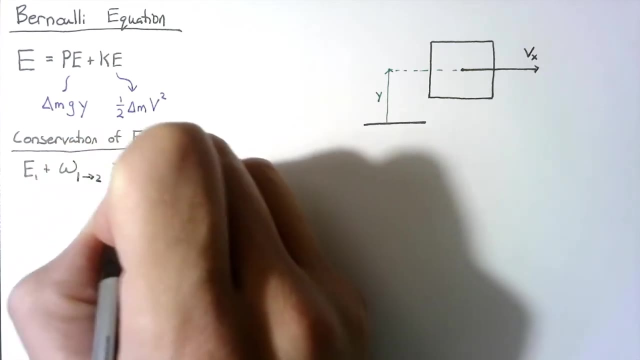 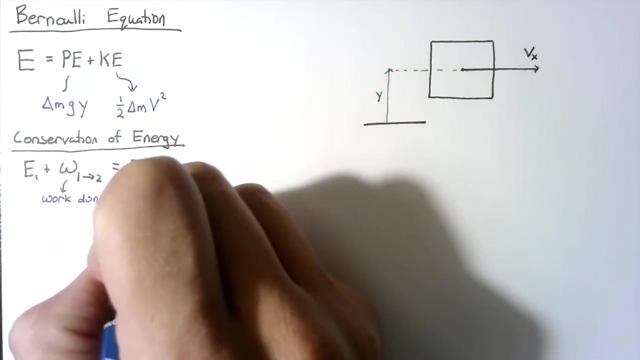 And all this says is that the energy at some state one, plus whatever work is done from state one to state two, is going to be equal to the energy of state two. Now, it's easy to have confusion about this work, but this is the work done on the element. 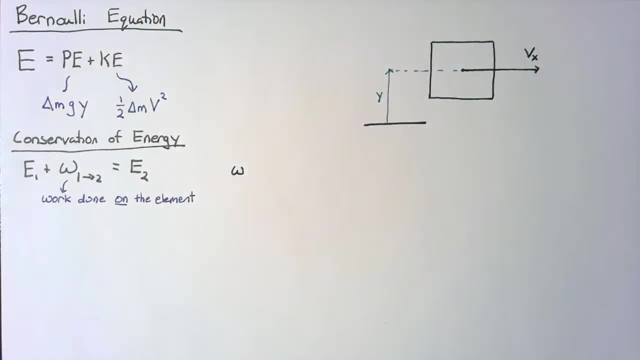 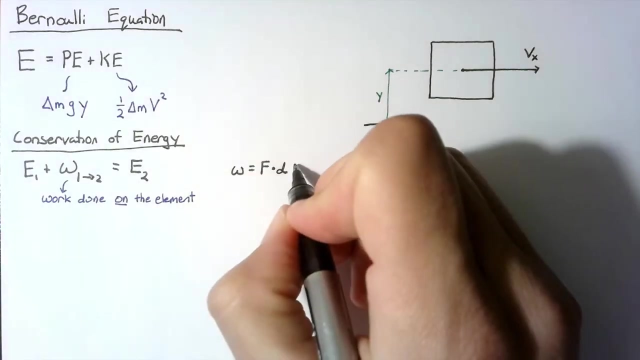 So now a reminder: work is simply the force multiplied by the distance in the direction that the force is occurring. We're interested in the total work for the element. We're going to work from one to two. So the way that we're going to write this is we're going to say that this is the integral. 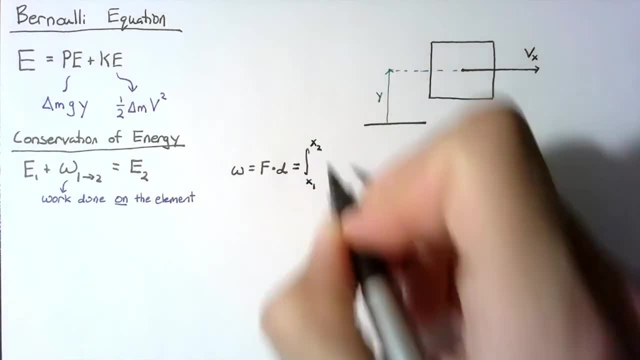 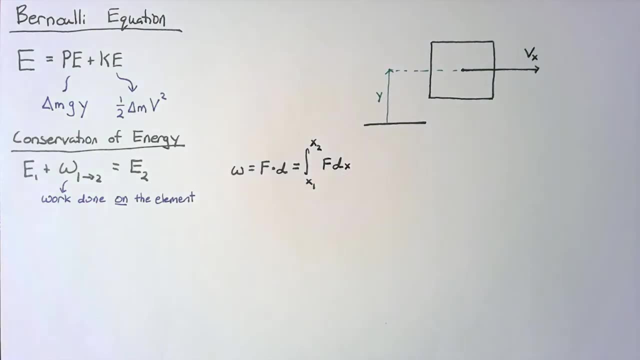 from some position x1 to some position x2 of the force multiplied by dx. That way if the force changes over time then we can keep track of that over the movement. We now need a position x that indicates how far along our particle is in the x direction. 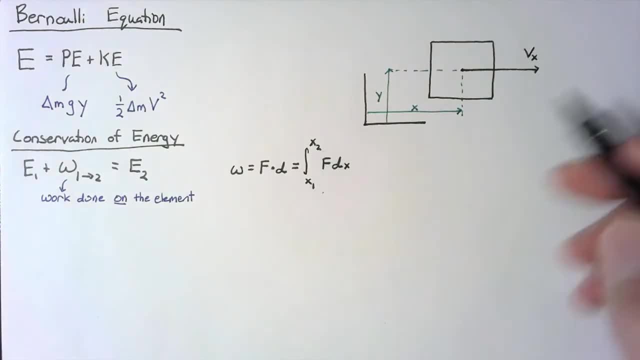 And since we're tracking the distance between these two states, we're actually interested in where this will be at some later point. So we're going to have two x values: One that we're going to call x1, that deals with the state one, and one at x2 sometime in the future. 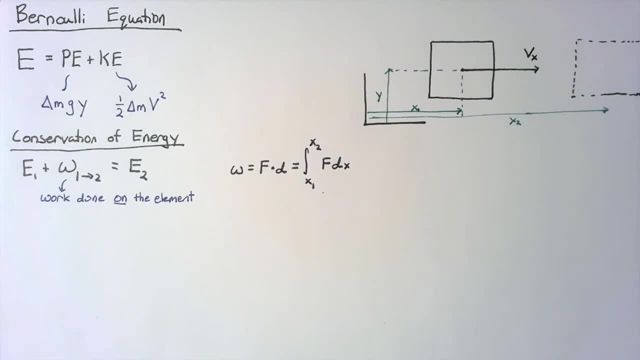 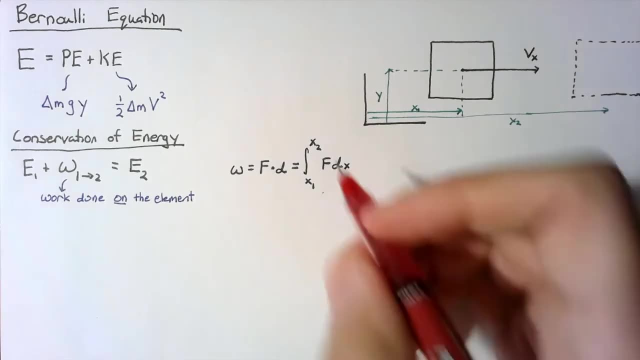 So between these two points, the position is obviously changing, but the velocity and the height and the pressure could all be changing as well. Now let's talk a little bit about this force. Remember once again, the force is just going to be equal to the pressure. 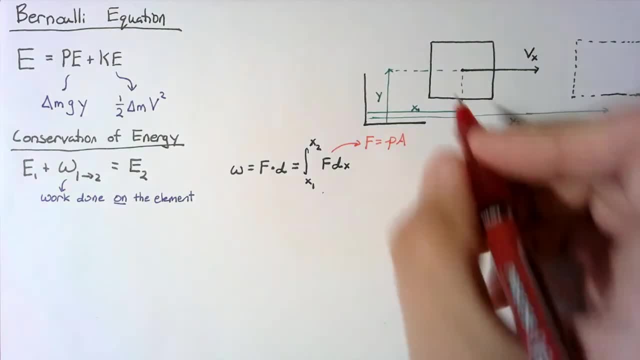 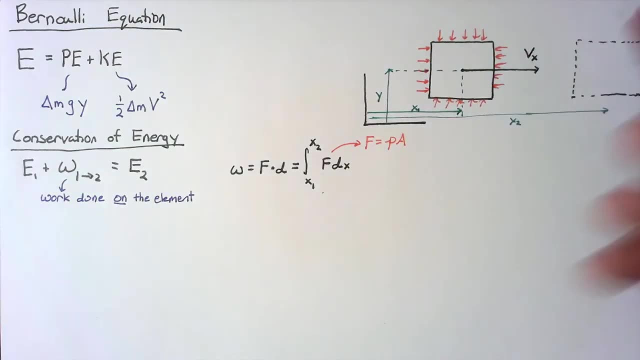 times the area of whatever surface it's pressing against. We're going to think about pressure acting on each of these surfaces, though, because we're only interested in the force in the direction of motion. we're really only going to track the pressures on the left and right hand sides. 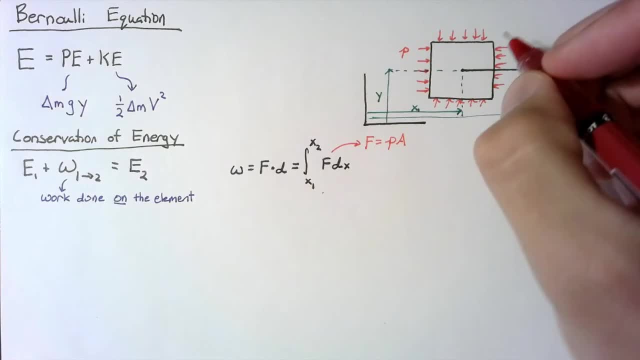 The pressure on the left side is going to be p, while the pressure on the right side is going to be p plus dp, dx times this delta x. So the total force here is going to end up being the integral from x1 to x2. 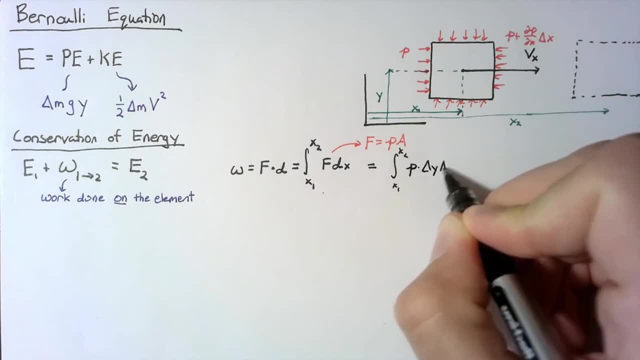 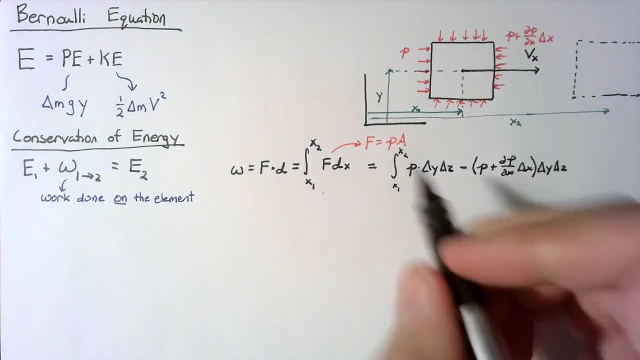 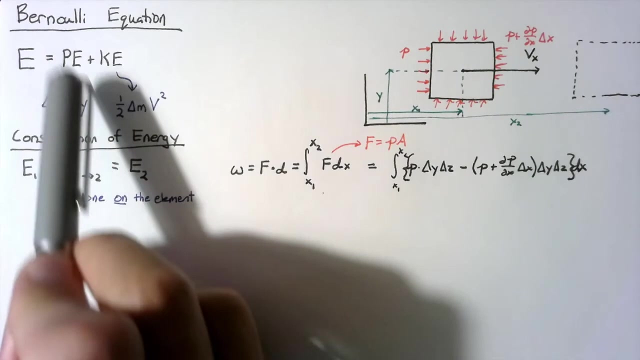 of the pressure times: delta y, delta z, minus this other pressure, again multiplied by delta y, delta z. All of that integrated in x. So now we have defined what's going on with the potential energy, kinetic energy and the work done. 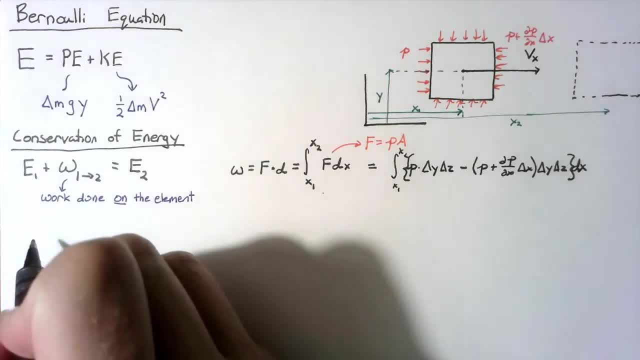 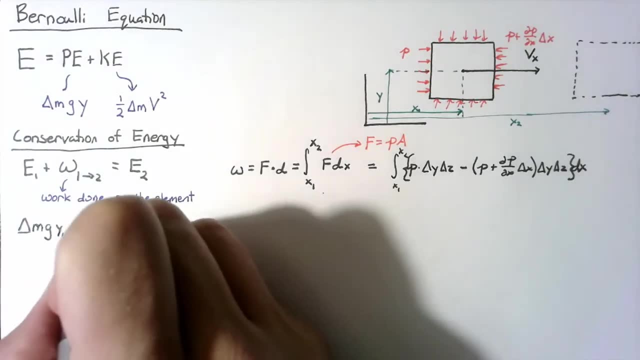 So we can write this out for both states. For state one, the potential energy is just going to be delta m g y1.. The kinetic energy is going to be one half delta m v1 squared, And then I can copy out all of this work. that's done. 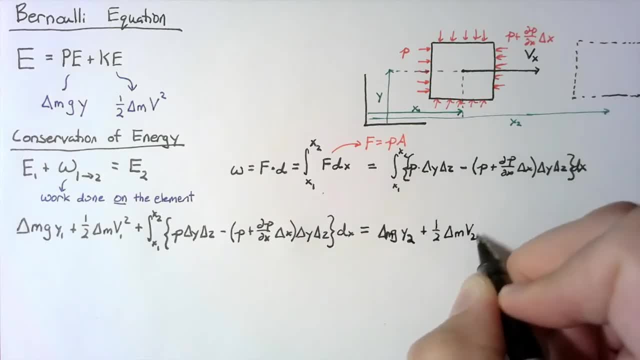 and that's going to be equal to the energy for state two. All that's left is the simplification of this integral, So we can get rid of the p's, which means that we end up with just a negative dp dx multiplied by the volume. 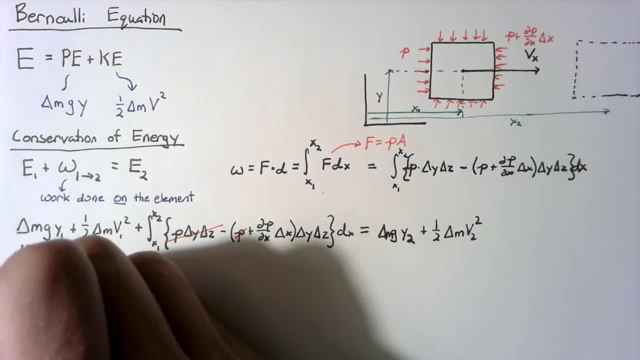 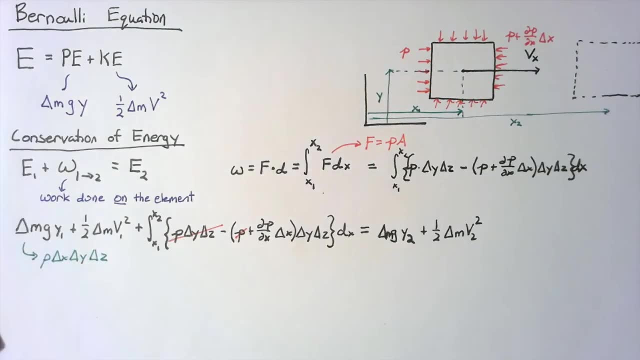 which we can take out of the integral. Keep in mind that this delta m is going to be equal to rho times, delta x, delta y, delta z, So we can actually get rid of all of the deltas here as well. Then these delta m's just become rows, and this gets much simpler. 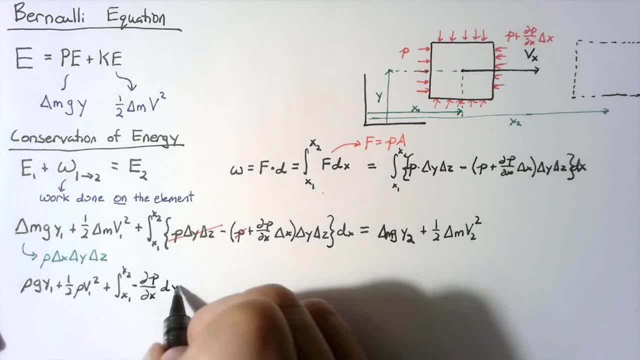 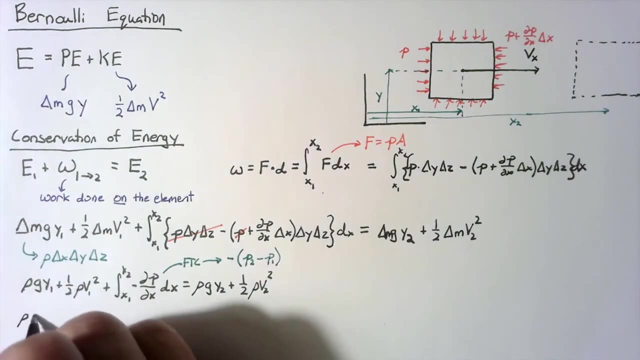 So let's rewrite that now. We can use the fundamental theorem of calculus in order to rewrite this as negative p2 minus p1. So we end up with rho g y1 plus one half rho v1 squared plus p1.. That's going to be equal to the exact same for state two.